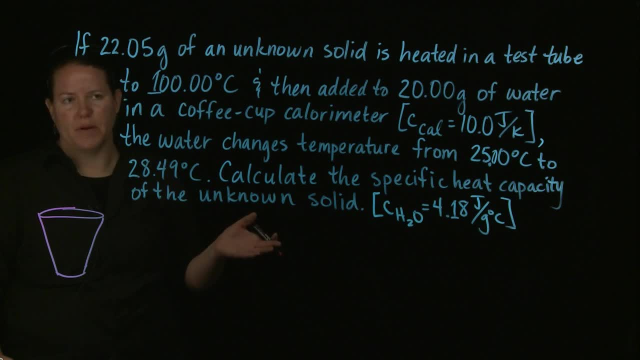 Okay, so in terms of thinking about it, that's why we call it a calorimeter. Okay, the real piece here is that we would love to use bomb calorimeters for everything. This is where calorimetry came about right. So, basically, in order to measure heat changes, you want to use a thermometer. 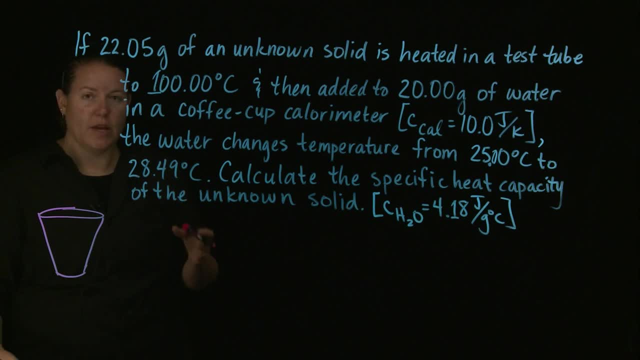 Bomb calorimetry was based off of the fact that you cannot use a thermometer if you're exploding something, because the thermometer explodes as well, And so because of that, We came out with this idea of having the heat transfer. Engineers really did a nice job, by the way, of figuring out a contraption in which the heat transfers very nicely from the exploding chamber. 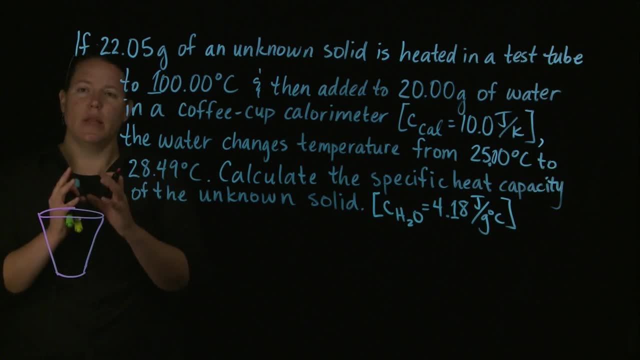 From the chamber in which whatever you're exploding explodes And the heat dissipates into water that is surrounding that chamber, And then you can measure the change in temperature of the water. So that's the basics of calorimetry. Coffee cup calorimetry is the same idea. 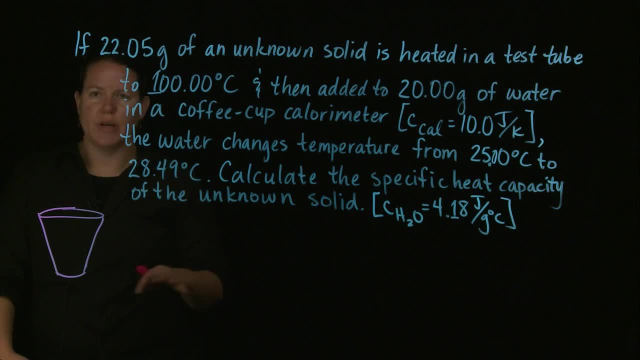 Except we can measure this with a thermometer, But you're still measuring heat changes a little bit indirectly. Okay, so there's my coffee cup calorimeter. I know that the C of the calorimeter is 10.0 joules per kelvin. 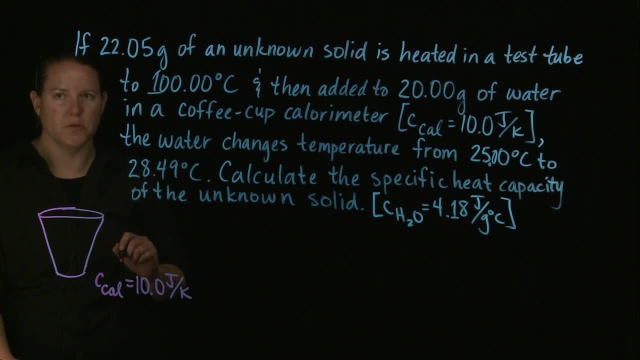 That's not joking, It's not texting language, It's joules per kelvin. Alright, And I know that I have in my lovely coffee cup calorimeter. I have 20 grams Of water And I'm forgetting a zero here. 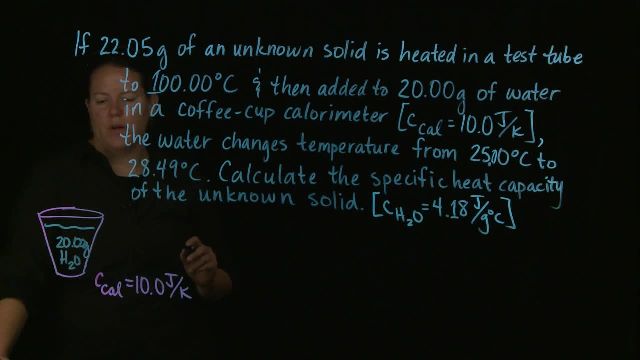 Woohoo, There's another zero. Okay, So 20 grams of water are in this coffee cup calorimeter. What's the initial temperature of the water? That's something to know. Alright, Do I have an initial temperature of the water? 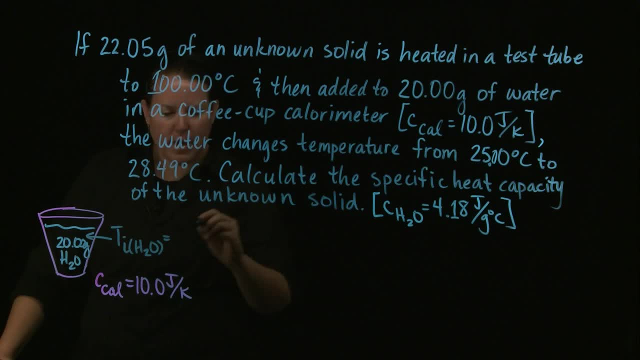 Indeed, I do. I know that the water went from 25.00 degrees Celsius To 28.49 degrees Celsius. So not only do I have an initial temperature of the water, I have a final temperature of the water. That is awesome. 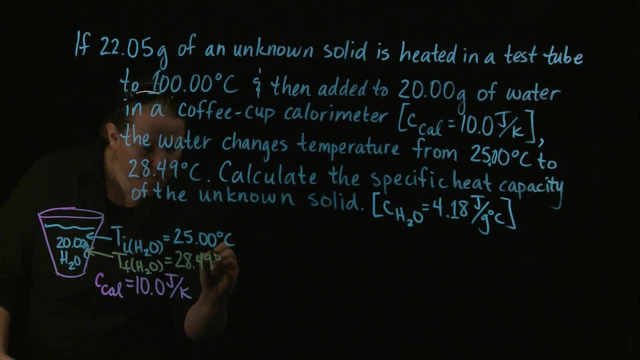 And a bit unexpected, Because sometimes that's the one you're looking for. Alright, Excellent. Where does that final temperature come from? Well, I heated some unknown Right, So I put: I put I have some unknown solid in a test tube. 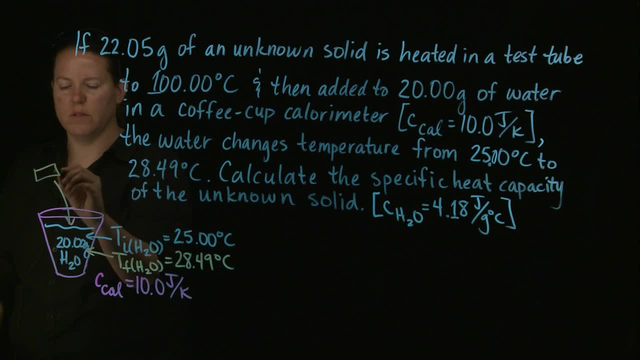 I'm just going to label the unknown solid Kind of like this: This is going to be my solid, Probably a crystal, I'm not caring, I'm just making some. But put it as a triangle, I don't care. 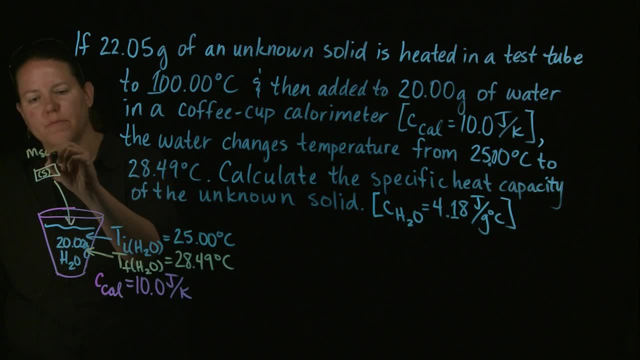 Just put it as something, Alright. So the mass of the solid is 22.05 grams, Right, And I know that it was heated in a test tube separately And then put in the water, So I know the initial temperature of the solid. 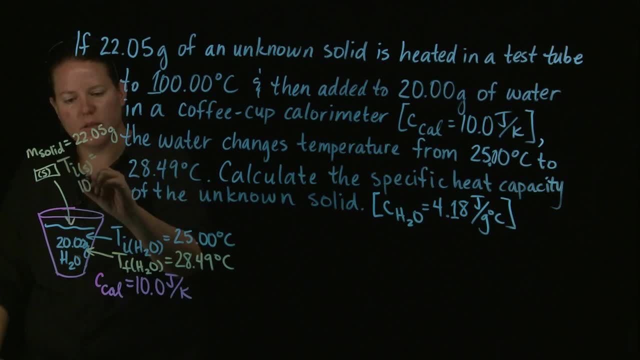 temperature of the solid is too, And that is 100 degrees Celsius. right, Alright. And then I don't know what the specific heat capacity of the solid is. but hey, you know what? I have one more piece of information: I have the specific heat capacity of water, which is usually given as a constant. 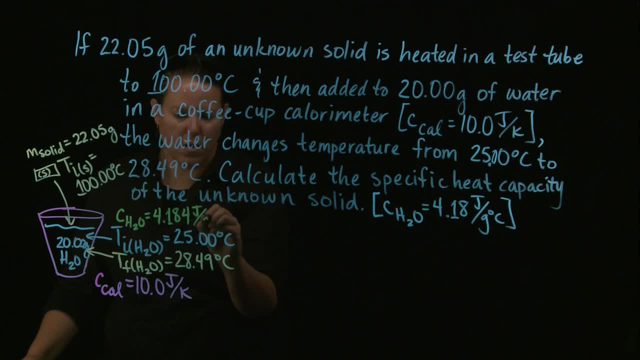 at the top of the test And I added the 4.. It's 4.184.. It's water again, as it often is, is the basis of the scales that we use, So everything else is based off of water. Water is one calorie. 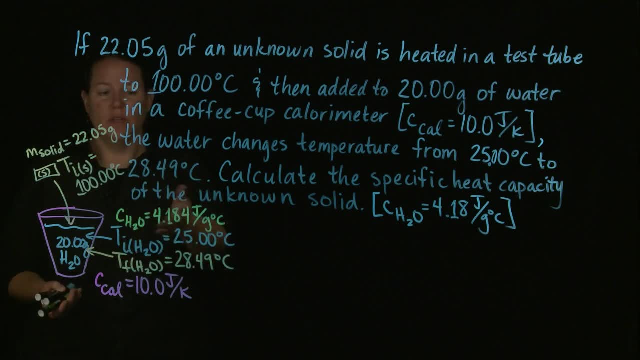 per gram degrees Celsius. Okay, so the conversion between one gram or one calorie and one joule is 4.184.. So that's why I'm adding a little bit there. Okay, I need to calculate the specific heat capacity of the unknown solid. Alright, so let's erase this And let's talk about what's. 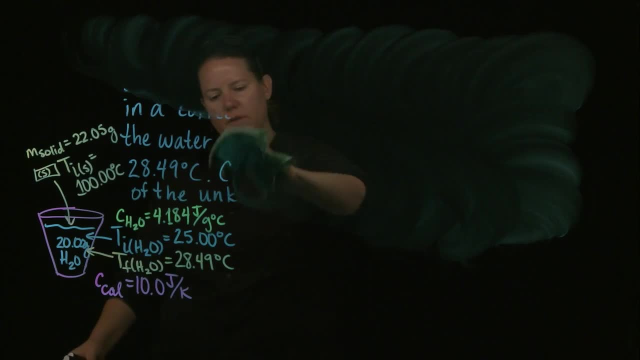 happening here. So my beginning question for you is: if you add hot metal or a hot solid to room temperature water, which is essentially what's happening here, Alright, so you add hot metal or a hot solid. often this is a metal here. i'm just saying it's a solid, hot solid. 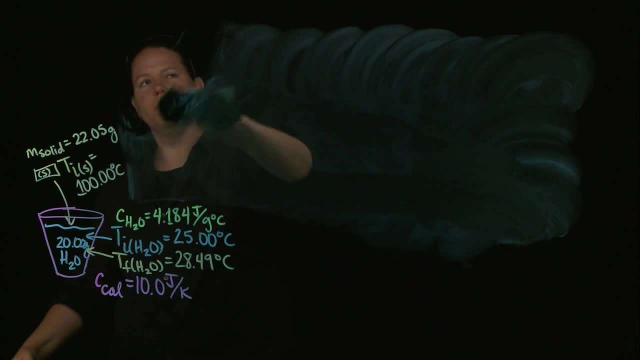 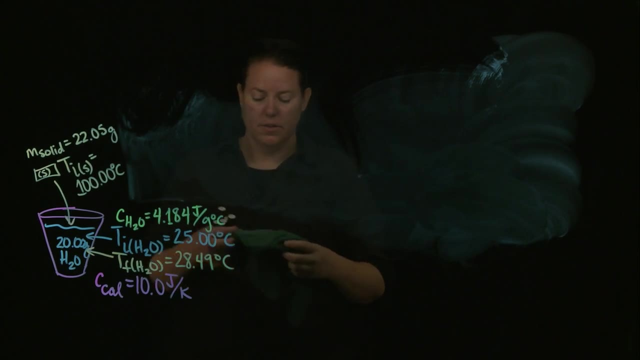 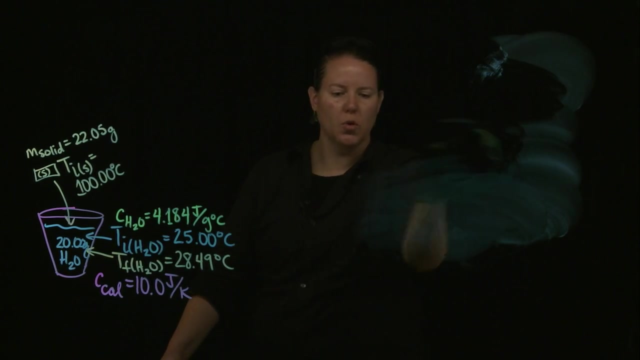 to room temperature water. what's going to happen, right? well, it should make sense that if you add hot solid to room temperature water, the water should heat up and the solid should cool down, and they should meet somewhere in the middle. does that make sense? because it should, right. so you add ice to a cup of water and the ice is cooler than the water is, and 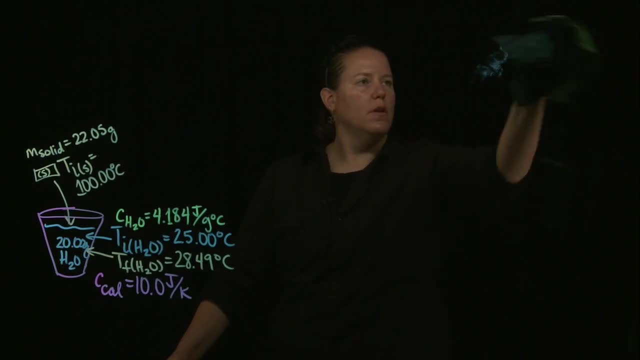 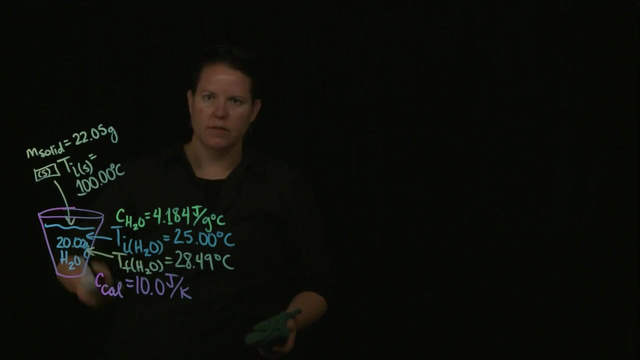 the water usually is at room temperature. you add ice to the water, then the water cools down and the ice heats up. it melts right. so in terms of this it's exact same thing, except in a kind of opposite way. this is hot, solid. you add it to basically cool water. 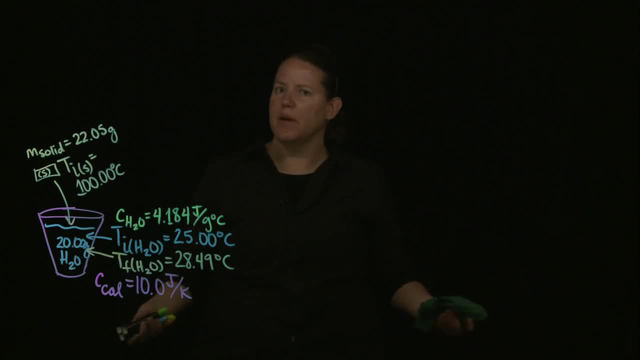 the solid cools down, the water heats up. they meet somewhere in the middle. so what's interesting here is that, while i said that the final temperature of the water is this value, it's actually if i put the solid in there, it's actually the final temperature of the water and the solid right. 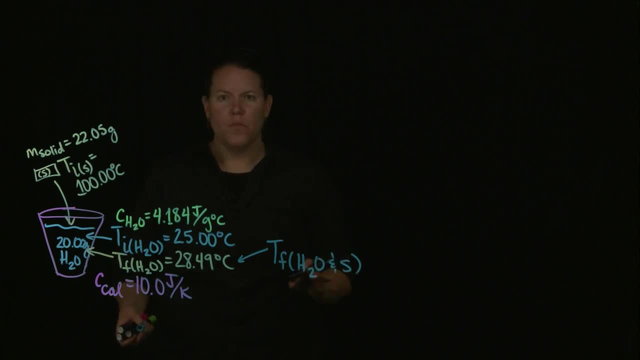 so it's for both. and then what am i making my uh idea here? what we would like ideally to happen is that you would have the solid and the water in the cup together and that no heat would escape the cup. so the point of calorific tree is that there's no heat coming outside of the cup. 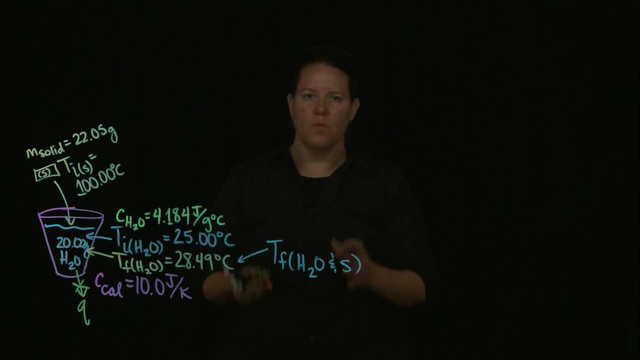 everything is contained within water and the calorimeter, or the cup in this case. Okay, so what I can say here? the formula for calorimetry is that the sum of the q's, the sum of the heats, is equal to zero. 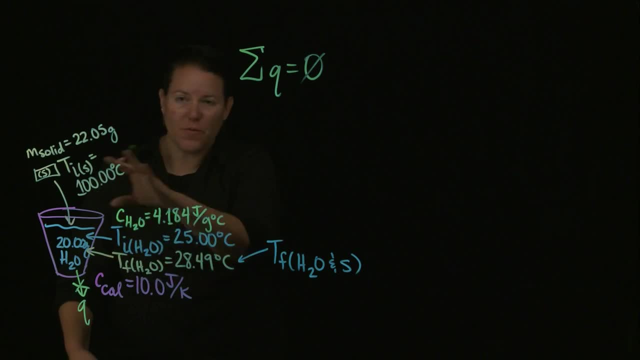 Okay, what I'm going to do is I'm going to identify a heat for each of these, right? So I have a heat for the solid, I have a heat that accompanies that solid, I have a heat for the water and I have a heat for the calorimeter or the cup. 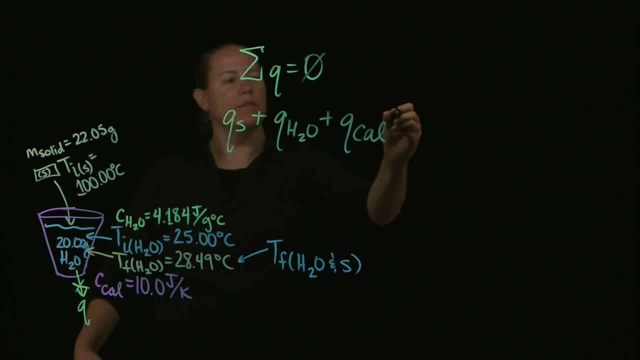 If I add all of those together, which is what the summation side means, then that should be zero. okay, Because basically this is all heats within the system I want the system to. I would like heat not to escape to the surroundings, okay. 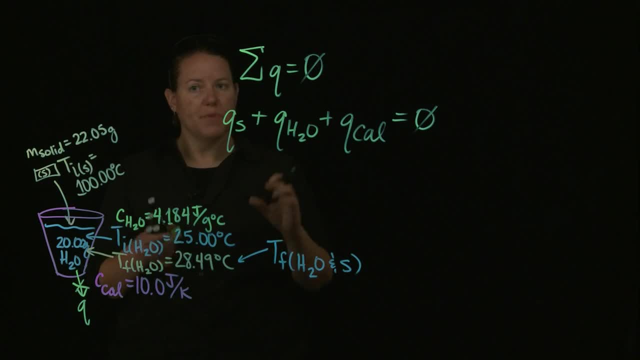 So basically, what I'm saying here is the system is enclosed and all of those heats can be added together and give me an overall heat of the system. okay, How am I going to find the heat of the solid? Well, I'm going to use the specific heat capacity equation, right? 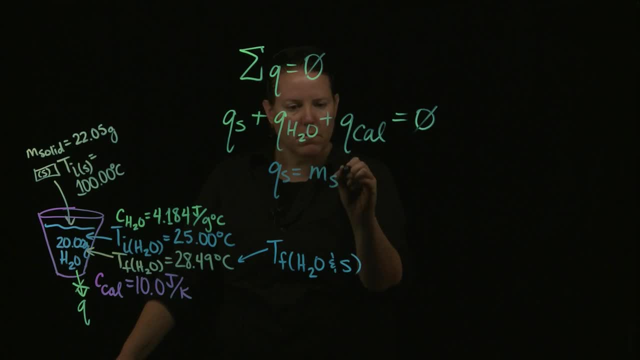 So that we know q equals mc delta t, right? So the q of the, the heat of the solid, is going to be equal to the mass of the solid times, the specific heat capacity of the solid times, the change in temperature, And q equals mc delta t is one of those equations you should just have on your card, okay? 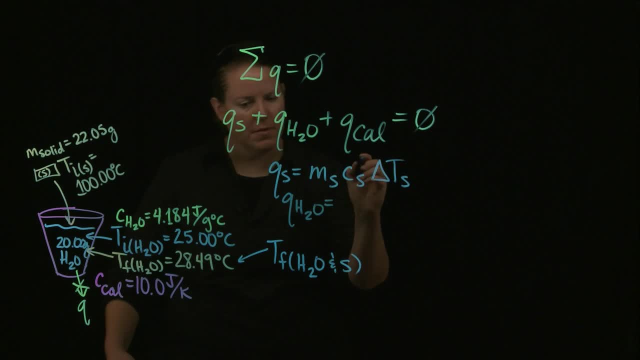 For exams or if you are given a card, you should memorize it right. The q of the water, the heat of the water is equal to the mass of the water. times, the specific heat capacity of the water times, the change in temperature of the water- all 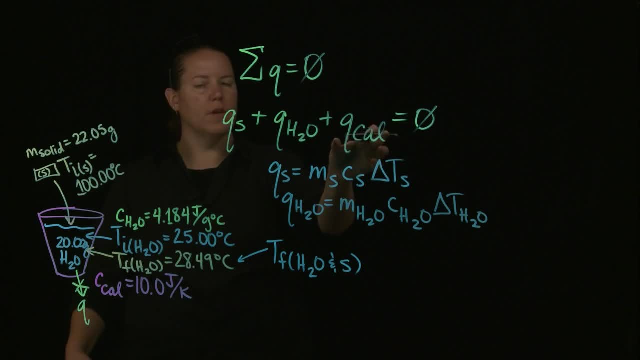 right, And not only that. I need the q of the calorimeter. What's interesting about a calorimeter is really its q is based Off of what you see in the specific heat capacity. So why is it mc, delta t for the solid and for the water? 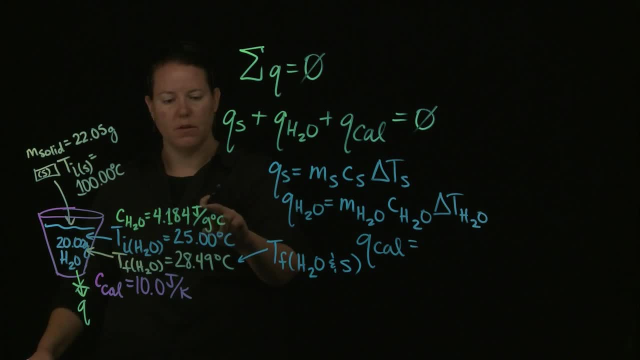 Well, look particularly for the water, where we have the specific heat capacity right. We know q is in joules, so there's joules right there. Mass is in grams. grams are right there. Change in temperature is in degrees Celsius. that's right there. 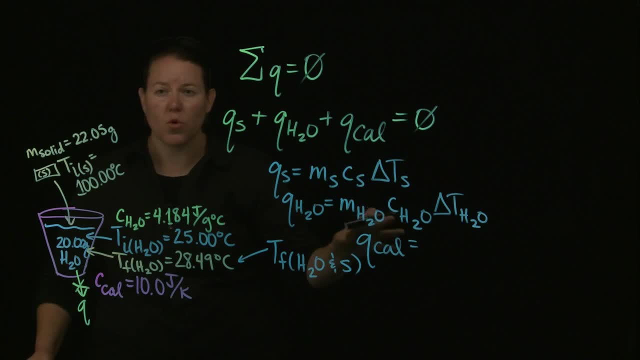 So, basically, my specific heat capacity is like my conversion factor. It's going to cancel out all the units that I don't want. Having said that, notice the difference Between the specific heat capacity of the water and the specific heat capacity of the calorimeter. 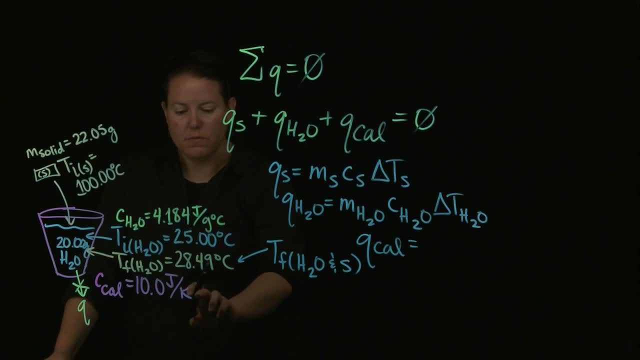 What's missing in the calorimeter's denominator right? That's a temperature value. Kelvin is a temperature value, But I don't have the grams, which means that the mass of the calorimeter we don't care about. We just don't even care. 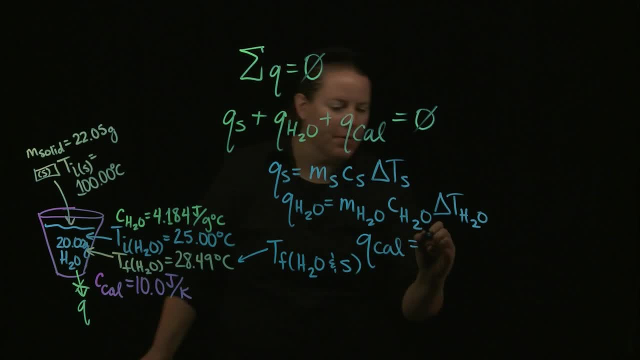 So therefore it would not have mass in the equation either. So the specific heat capacity of the calorimeter Times the change in temperature of the calorimeter. The assumption here is that the change in temperature the water is lining the cup in its entirety. 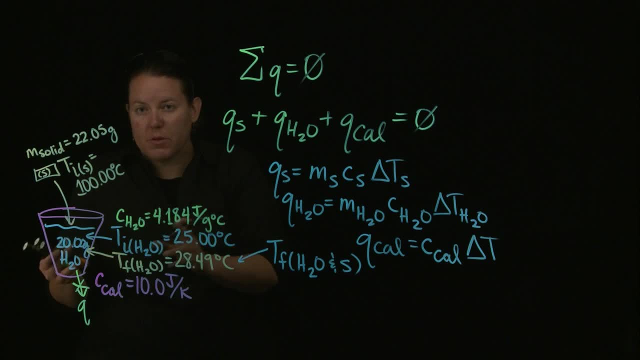 So, because water is lining the cup in its entirety, the change in temperature of the calorimeter. Let me write this down: The change in temperature of the calorimeter is the exact same as the change in temperature of the water. Those are equivalent values. 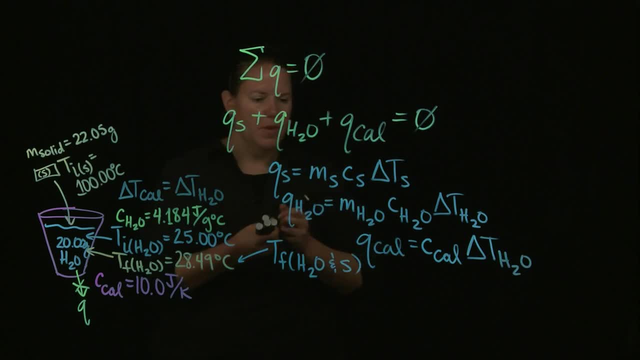 And so I'm going to put that right here. All right, So now I need to put this all together. Just a little bit of something. I have all of the values for the water, So I should put all of those in right. 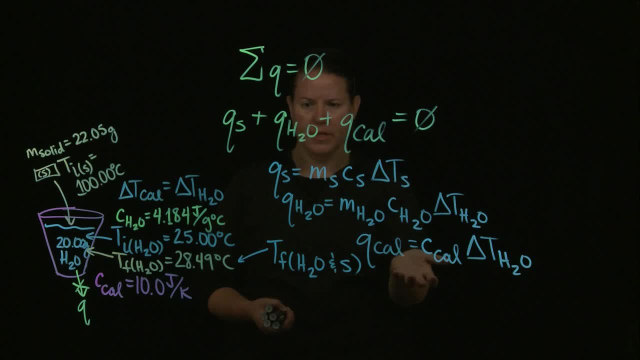 I have all the values for the calorimeter. I should put all of those in. But what am I missing out of the Q of the solid? I'm missing the specific heat capacity of the solid. If you remember back to the problem, that's actually what the problem asked for. 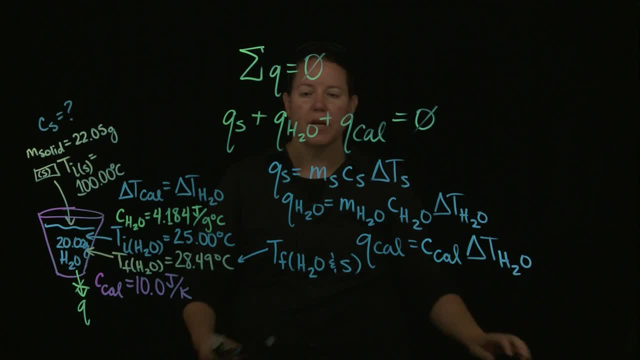 It asked for the specific heat capacity of the solid. So Because of that I need to maybe plug in my numbers here, put them in here. but then I need to keep the solid, the Q of the solid, on its own side so that I can solve for C. 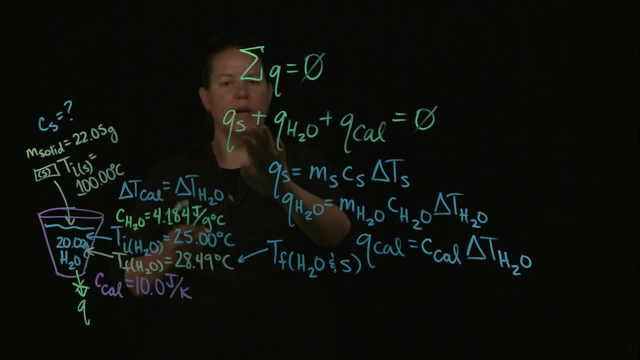 Okay, So I'm just going to modify this formula a little bit. I'm going to keep, I'm going to basically isolate or solve for Q of S. And by solving for Q of S, If I put the equal sign here, I need to subtract both of these from both sides. 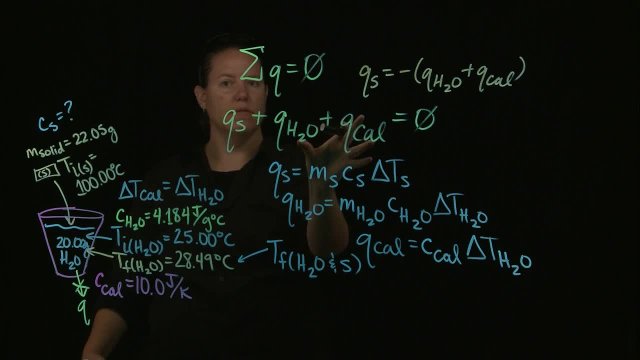 When I subtract it from this side, it goes to zero. When I subtract it from this side, then I just get those values. Okay, All right. And the reason why we did that, just to reiterate, is because we needed Q of S alone, because 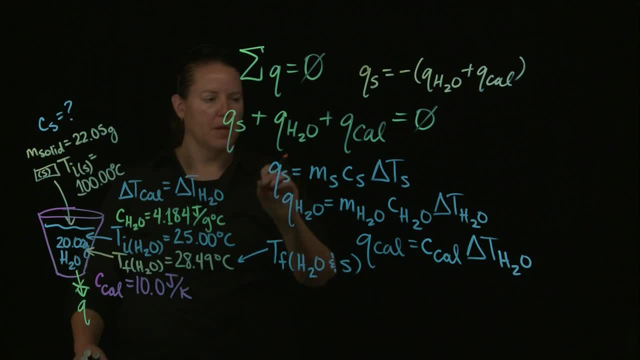 what we're looking for is in the midst of Q of S. Okay, So let's plug in our numbers. for Q of water, The mass of the water was 20.00 grams. Can you guys see this? You guys can see this. 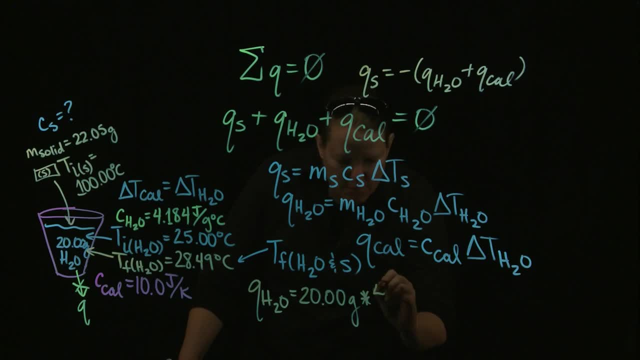 All right, Good Times. the specific heat capacity of water, which is 4.184 joules per gram degrees Celsius- Remember I added a four here from the problem Doesn't matter. All right, And the change in temperature of the water is 28,. is the final minus initial. 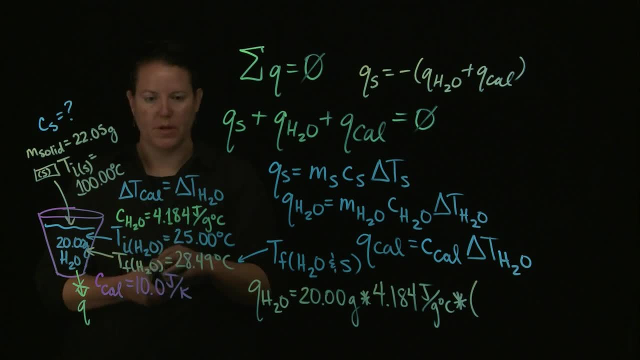 So let's maybe do that over here, because we're going to use it for two different values, right? So the change in temperature of the water, delta T of water is equal to the T final of the water minus the T initial of the water, which means that I'm going to do 28.49 degrees Celsius. 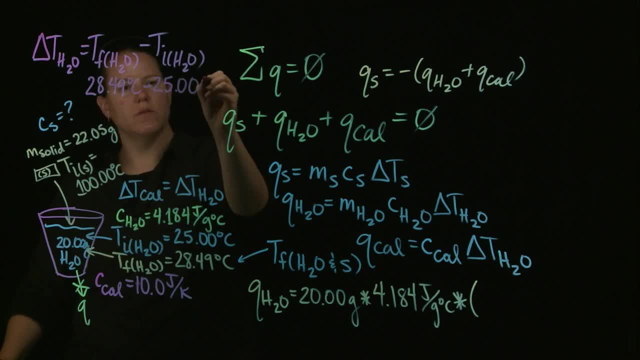 minus 25.00 degrees Celsius, which means that the change in temperature of the water is equal to the T final of the water. So that is going to be equal to 3.49 degrees Celsius, right, And I can insert that for change in temperature of the water. 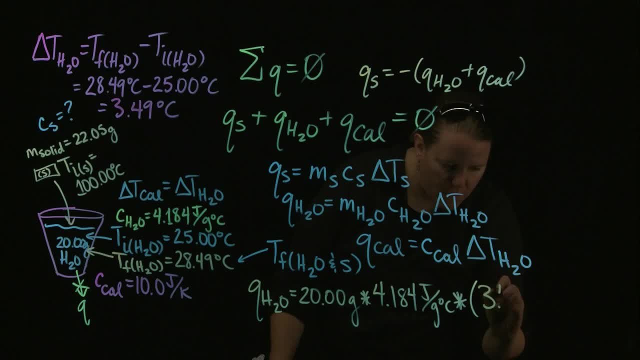 So let's put that over here: 3.49 degrees Celsius. right, I can do the Q of the calorimeter as well. Let me actually multiply this out. So 20 times 4.184 times 3.49.. Equals 292.0. 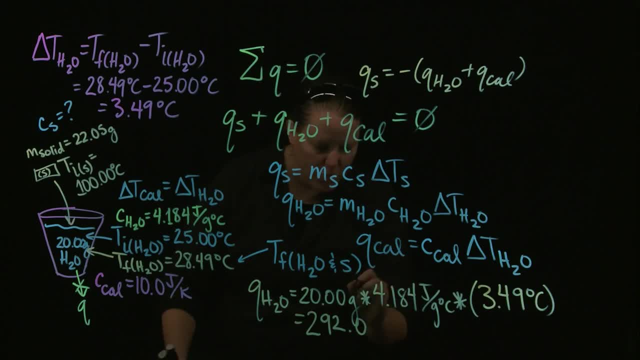 And notice that grams canceled out. Just as we said, the conversion factor is specific heat capacity. here Grams on top and on bottom, they cancel out Degrees. Celsius cancels out, which leaves me with joules alone in the end for the water. 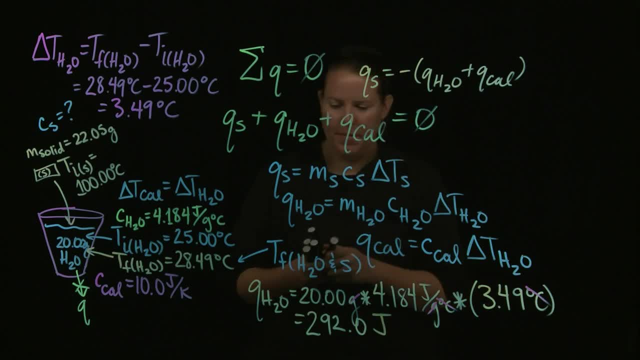 Okay, I need to do the same thing for the Q of the calorimeter. The Q of the calorimeter. I'm kind of losing board space here, So we'll do it Really really quick right there. All right, So the Q of the calorimeter was 10 joules per Kelvin. 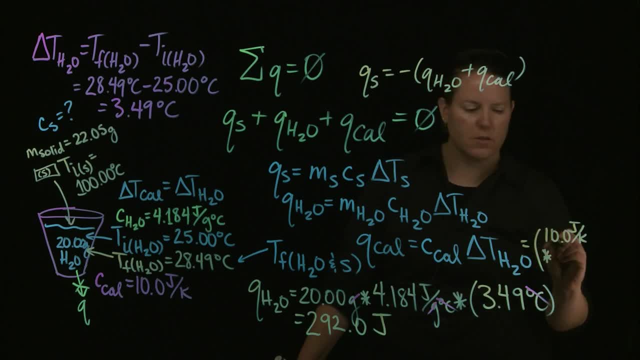 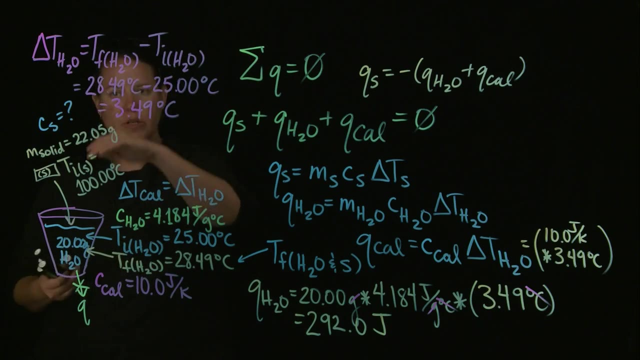 And the change in temperature of the water is 3.49 degrees Celsius. So now your question is: can degrees Celsius and Kelvin cancel out? And of course they can. in this particular case, Remember that we're taking a change in temperature, And changes in temperature for degrees Celsius and Kelvin. 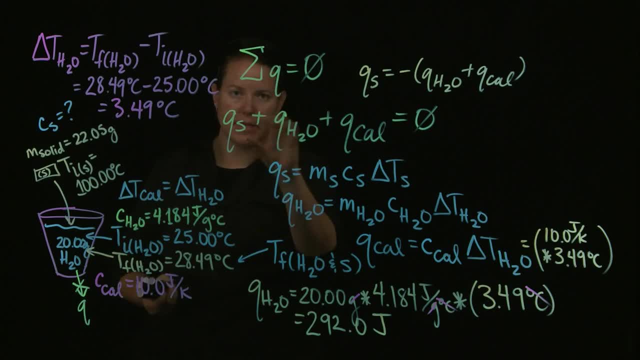 are the same. Okay, Why is that? For just a quick moment, Because you would add in 273.15 to this particular value for degrees Celsius. And you would add in 273.15 to this value of degrees Celsius, Which means that when you add it in, because you're subtracting this whole entity. 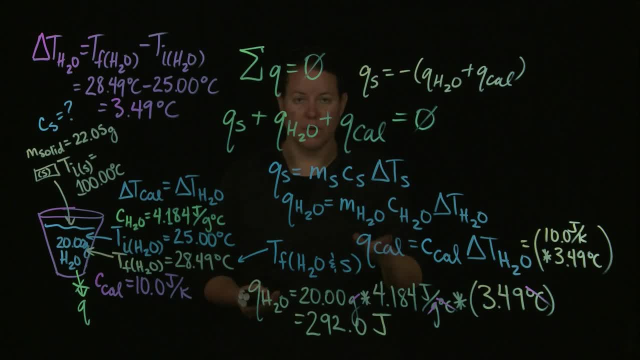 you would then subtract it back out. Try it out, guys. It comes out to the same exact value. So because of that, I'm going to just degrees. Celsius and Kelvin are going to cancel out And my Q of my calorimeter that I'm going to write right here. 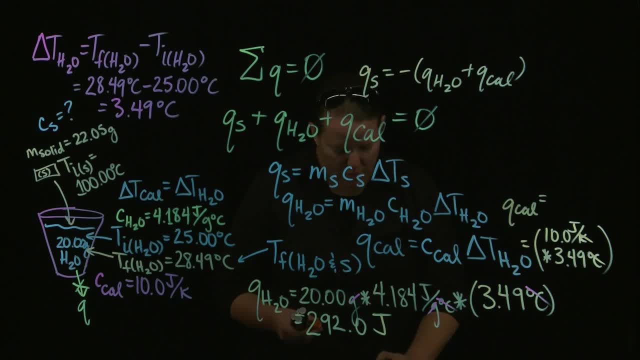 is going to be 10 times 3.49, which I'm pretty sure is 34.9.. But you know it's good to double check Joules as well. Okay, Now I can plug that in right here. 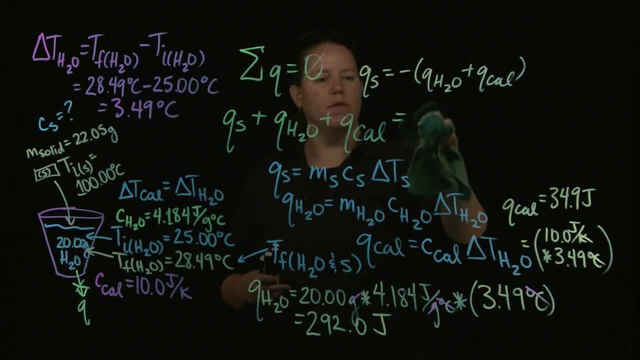 So let's go ahead and do that, Let's erase some of this stuff, At least this line, So that I have a little bit of room to work. Okay, Alright, So When I plug these two values in, And, by the way, if you're never given a C of a calorimeter, 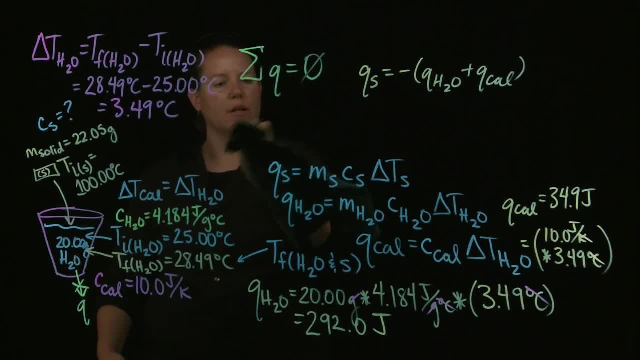 okay. so if you're not given the heat capacity of the calorimeter, then we consider it to be negligible. Negligible is just saying: look how much heat was contributed by the calorimeter versus how much heat was contributed by the water. 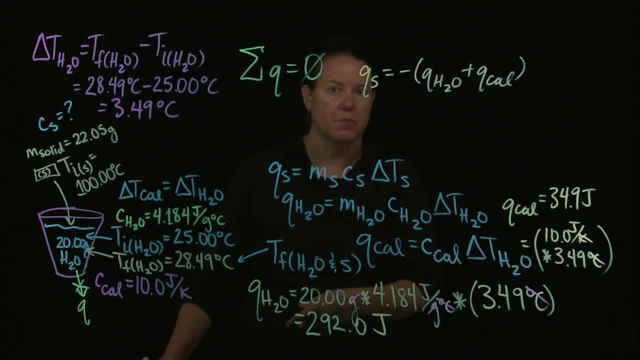 It's like a fairly big difference, And usually it's even smaller than this. This is way smaller than this, So we can basically say that it doesn't count. But if you're given the specific heat capacity or the heat capacity more specifically, 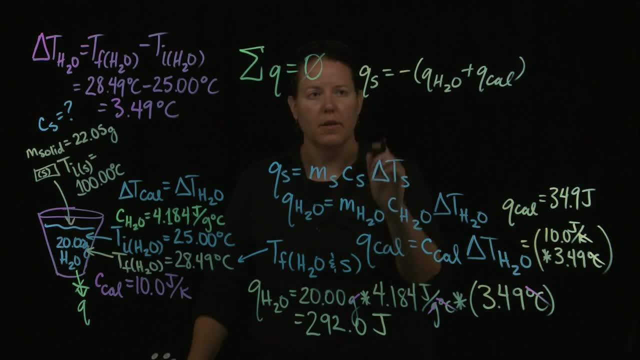 if you're given the heat capacity of the calorimeter, then go ahead and calculate this Q. The Q of the solid is going to be equal to water: 292.0 Joules plus 34.9 Joules, And that's going to be equal to. 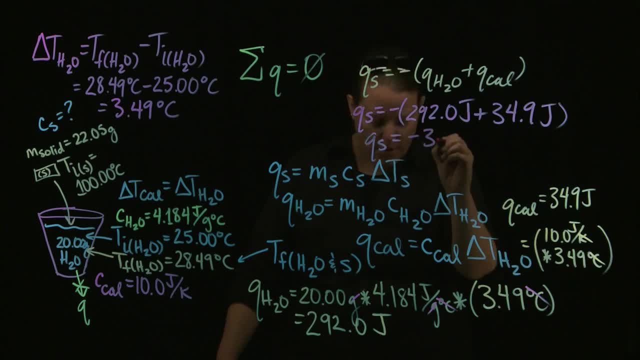 negative 326.9 Joules. Perfect, That's an excellent place to be Now that we're here. what we would really like to do is we would like to use this equation and plug this in, right? So let's erase all of this stuff. 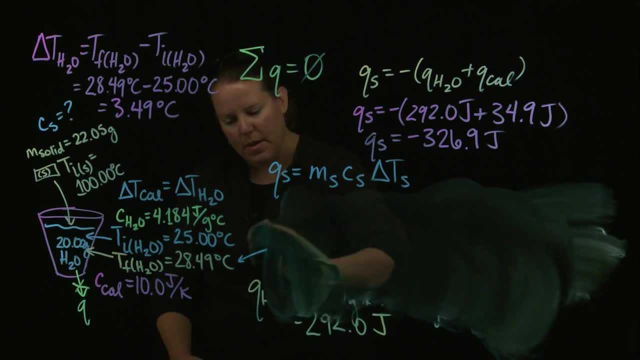 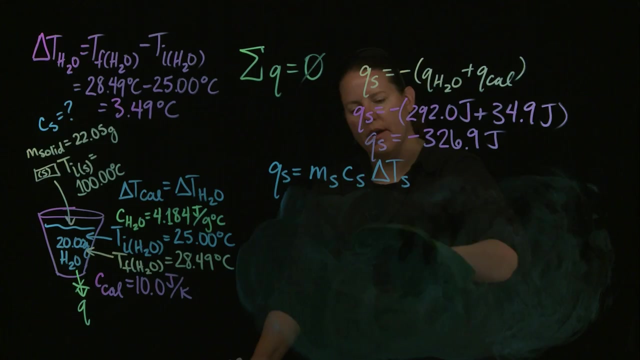 underneath here And we'll get to work solving the rest of this right. So, in terms of dealing with this, you're going to have an ability to identify the unknown solid if you had a list of specific heat capacities of the unknown solids, right? 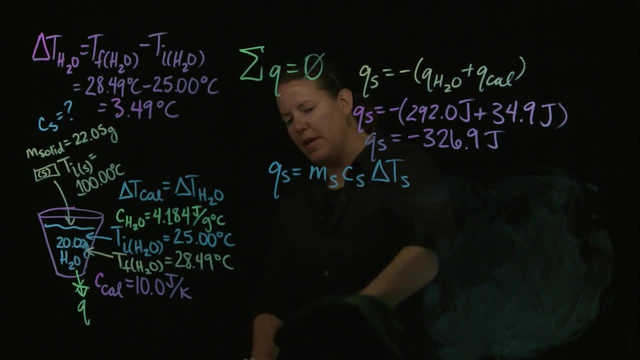 So if we knew what the specific heat capacity ends up being and we could then go to specific heat capacities that are known and compare and identify Right. Some metals have very similar specific heat capacities, so you probably would have to be given a list. 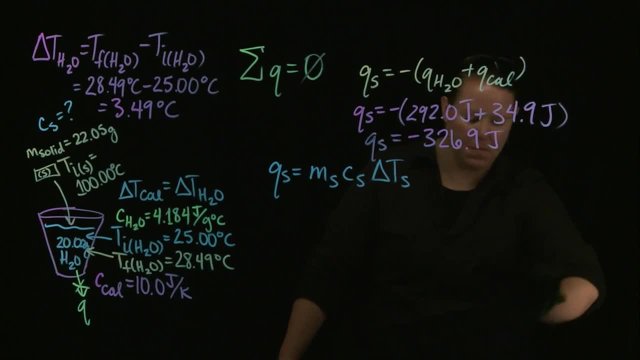 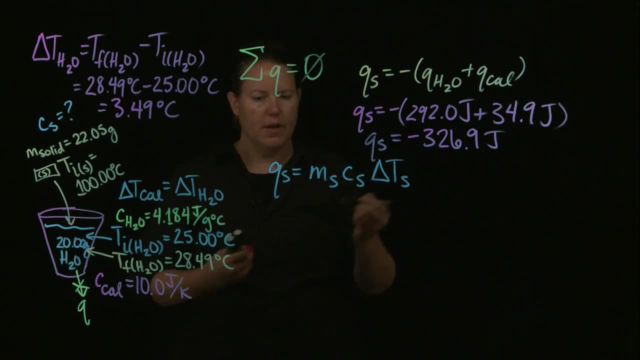 of those that were used in the experiment, And hopefully they would be fairly different from one another. Alright, So now that I have Q of S, I have this. I need to solve this equation for C of S, because that's what I'm looking for. 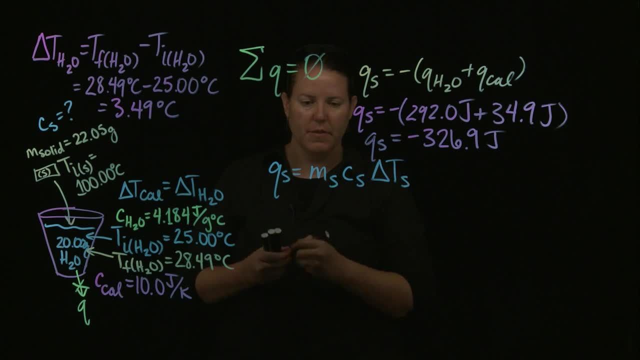 If I want to solve this equation for the specific heat capacity of the solid, remember I need to get it alone on one side and in the numerator. It's already in the numerator, so I just need to get it alone. I divide both sides. 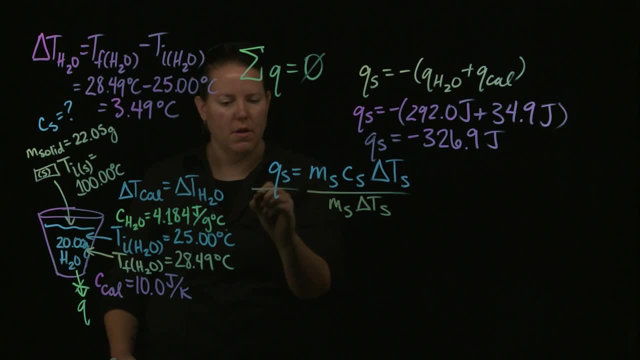 by whatever's around it. and lo and behold, these cancel out And I get C of S, or the specific heat capacity of the solid is equal to the Q of the solid divided by the mass of the solid and divided by the change in temperature of the solid. 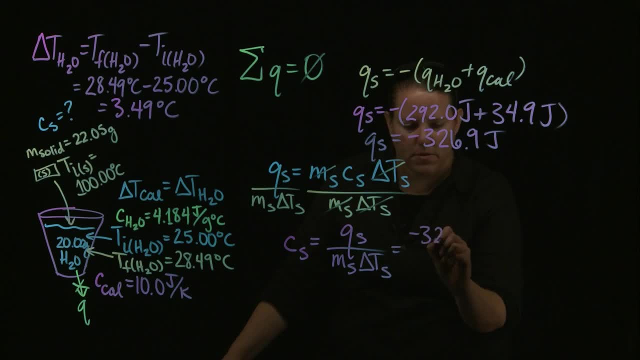 Here I have my values right. So negative 326.9, joules Mass. here is. let's go back over to my picture. the mass of the solid was 22.05 grams and the change in temperature of the solid. 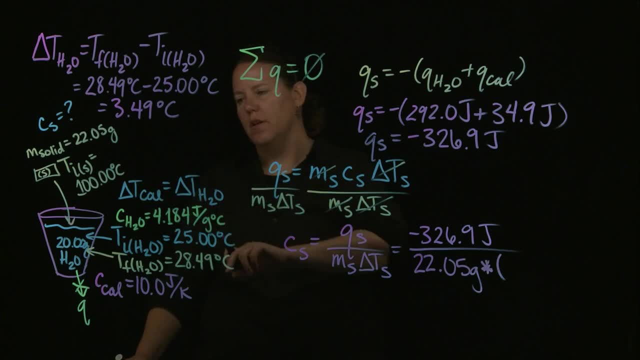 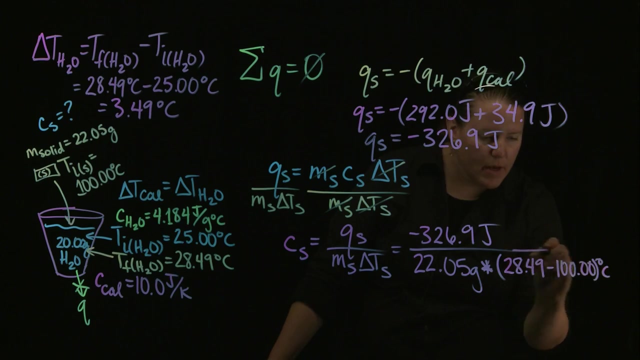 let's look at that for a moment. the change in temperature of the solid: the initial was 100, and the final of everything was 28.49.. Which notice? this gives you a negative number. This difference is a negative number.